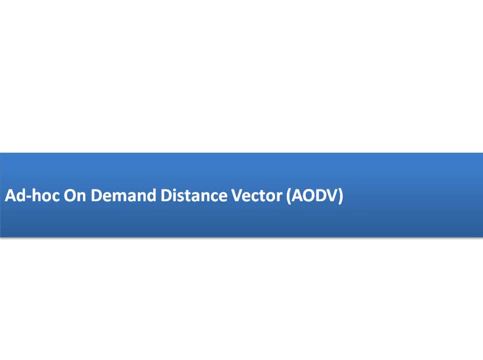 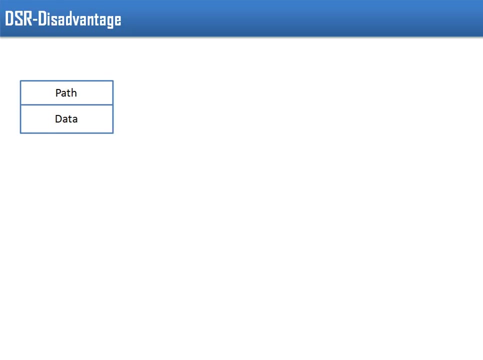 say this is the extension of DSR, dynamic source routing. so before going for AODV, just have a look on DSR disadvantage. so in case of dynamic source routing, whenever a node finds out a route to the destination, the path will be included in the data. 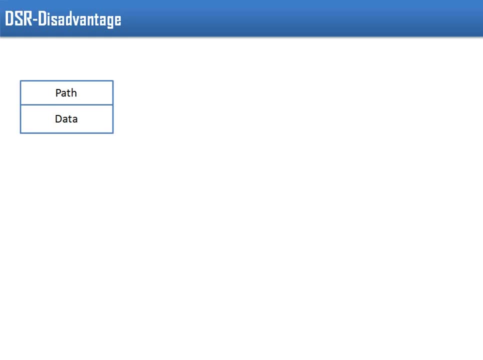 itself the data packet carries the entire route. so for example, say: if our network is not large, so path will be small, but if our network size will grow, so in that case the bytes required will be small, so in that case the bytes required to store path and data packet will also increase. so most of the time in this 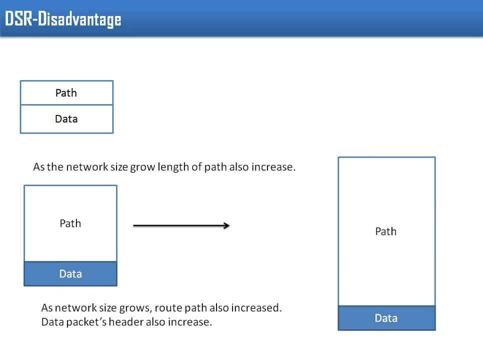 case, network bandwidth will be not used, not utilized fully, because most of the time most of the bandwidth is used to send path across the nodes. so this was the first disadvantage. the second one: in DSR, for one destination, there are multiple route possible. one node can cache multiple route for. 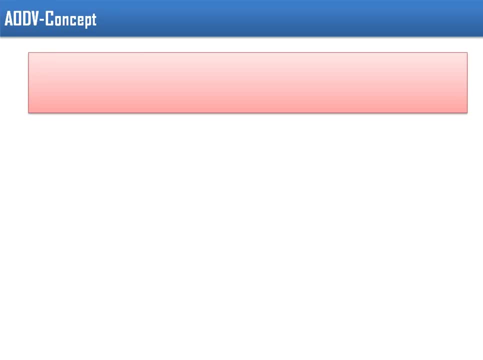 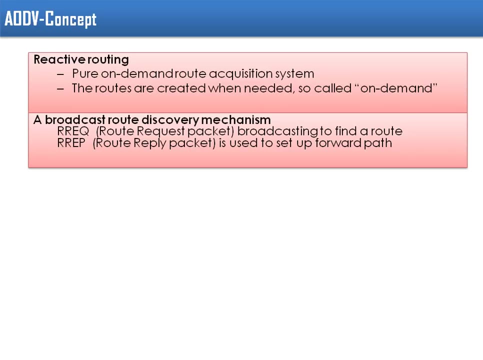 the same destination. so in AODV- AODV reactive routing protocol- the route discovery mechanism is similar as we are having in dynamic source routing. so this: in order to discover a route first, it will send a route request packet. when the destination received that packet they will reply by sending route reply packet. we will see this example. let us slide. 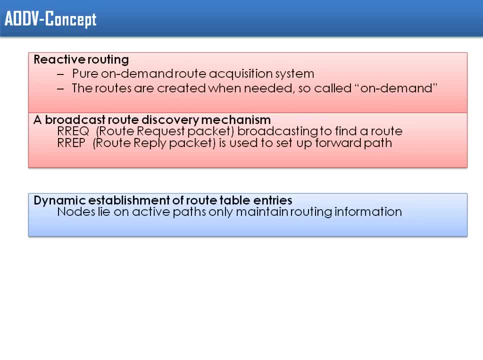 now AODV maintain all the route in the form of table, where in DSR tables are not used, but here we are using table. AODV routing protocol store all their path in form of table. now, when we have, when any entry made in table, one timer also. 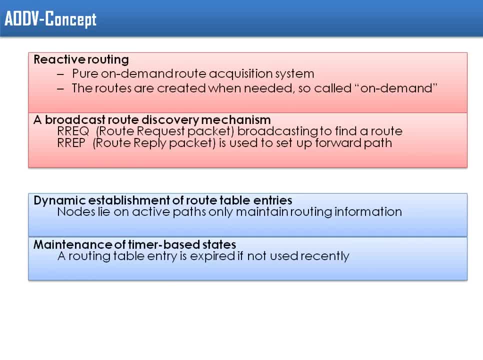 associated with that tables. that timer will explain, sorry. that timer will specify at what time that entry should be removed from the entry. sorry from the table. and the third one is the destination sequence number. destination sequence number: it can be considered like a timestamp, so at what time we have received this path information from the destination. so in 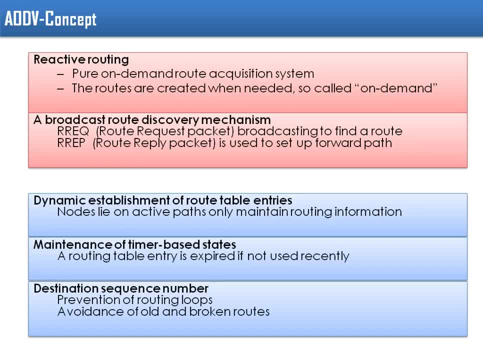 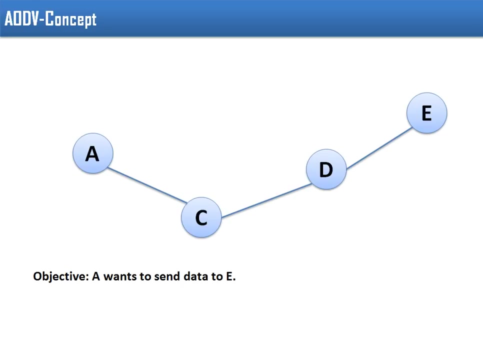 case of if the information is old, the information is not fresh, information is still. in that case the destination sequence number can be used to check whether that coming information is fresh or not. so inclusion of destination sequence number also avoid routing loop account to infinity problem. so let's take an example. we are having four nodes: AC, DE. 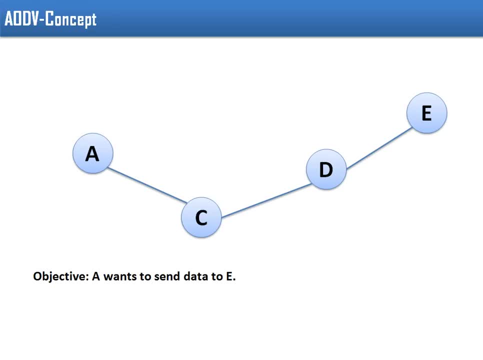 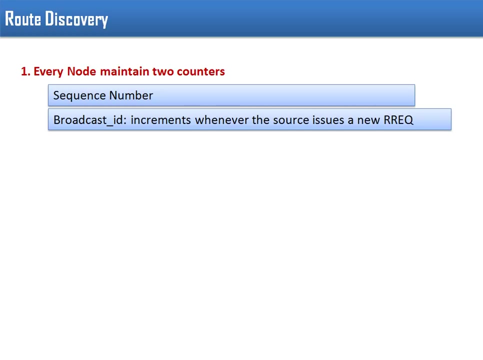 our objective. A wants to send data to E, so in which is the node is not having any information. that where is that not being not E exist in the network? so he will start a route discovery mechanism. so they will send their sorry, they will broadcast the route request packet. so in 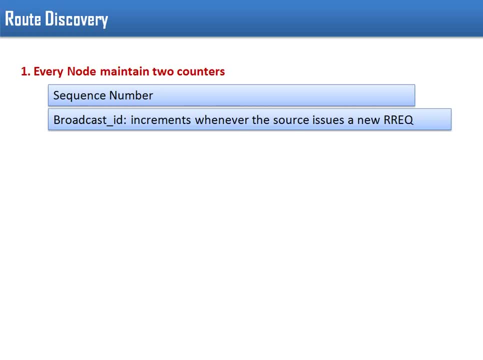 route request packet. all entries are same as we are having in DSR, but there are some changes, so every node maintain two counter. one is sequence number, so the sequence number will work as a timestamp, and second one is the broadcast ID. whenever any node send a route request packet, that packet carries a unique ID, so that broadcast ID. 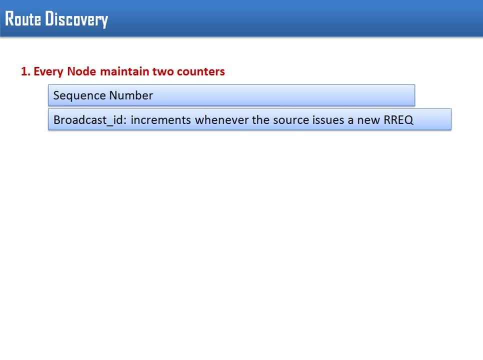 every node maintain. whenever they send route request packet they increase this ID. so next time when they will send route request packet, that will be having another ID. and this is the packet format for route request in AODV. so first entry is the source address, second one is the source sequence number. so when 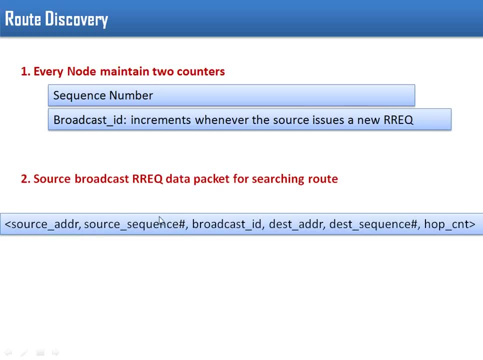 source will generate this packet at the time. they will include their sequence timer information, their sequence timer current value and this is the broadcast ID. this is, we can consider, you say, unique ID for route request packet. then this is the destination address, destination sequence numbers. if sender is not having any idea about destination, so in that case this: 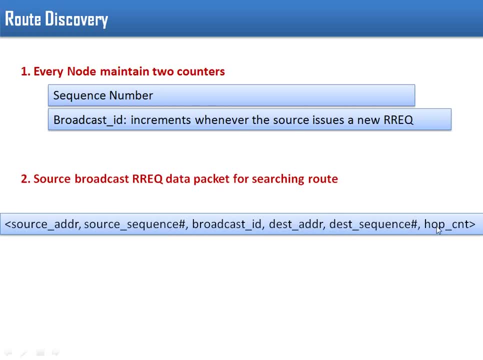 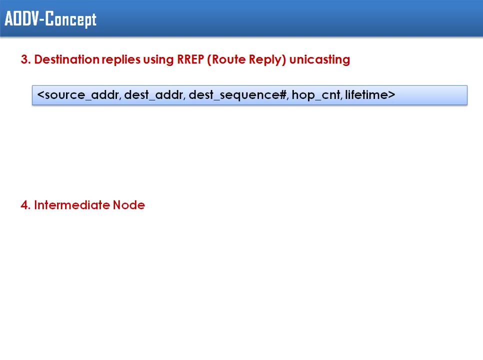 entry will be empty. and the last one is the hope count- how many hope it's required to send data from sender to receivers. so when destination receive route request, it will check the destination address and it will find out that this route discovery process is for its own. so 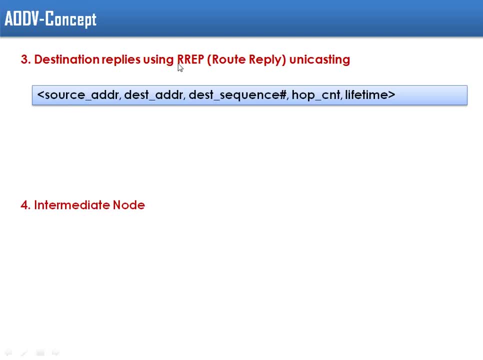 in that case destination will reply by using route reply packet. so the format is source address, destination address, destination sequence number. so now, when destination will send this packet, they include their timestamp, hope, count and this is the lifetime. this will specify for how long this entry, this path, can be used. 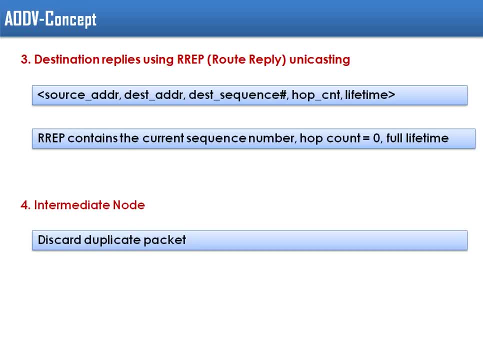 intermediate node. so intermediate node- whenever they hear duplicate packet, they will discard it. now in case if a sender is requesting for a route, they will broadcast in the route request packet in case if intermediate node having any updated information. so in stead of broadcasting route request packet, they will send a reply to the sender. 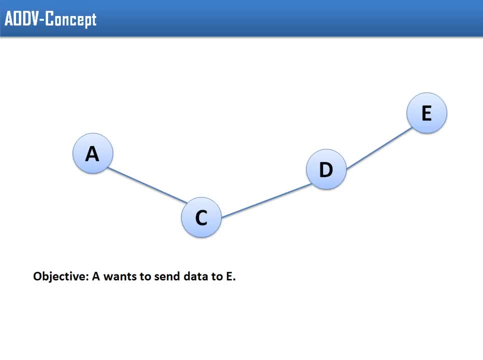 so now let's continue our example. so he wants to send some data to e. so A has to start a route discovery process. so under this process, a needs to transmit route request packet, so that packet we are considering here. so first one source address, source sequence number. this is the destination sequence. sorry, this is the destination. 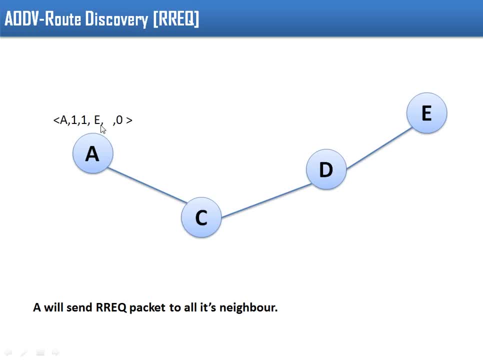 address, destination sequence number: this is the hope count and this third unit is the broadcast ID. so we are assuming all these value from the initially these are value this node is having initially this hope count 0. this hope count actually signify the distance from the Sanders. so initially we are at node a. so between 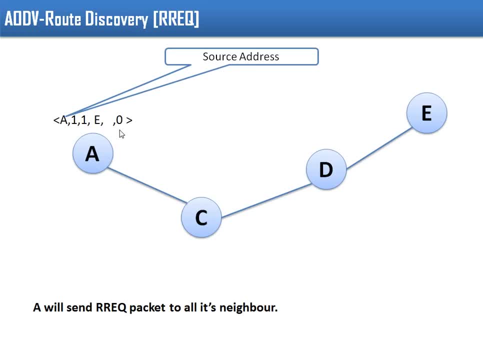 a. 2 is 0, so now A will broadcast this packet. so these are the meaning of these. were wifi got you, so they will send. it will broadcast this packet. A is having only one neighbor, so this packet will be send to C. now C is not having an. 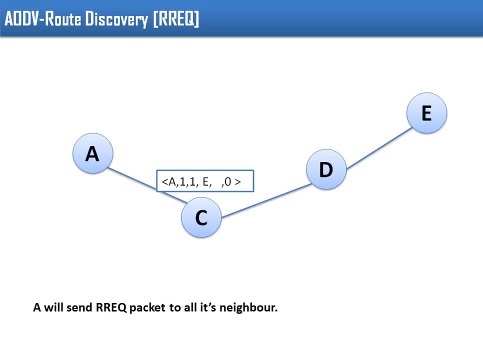 information about node E. so C will broadcast this packet again. now, before broadcasting this packet, C will update this hope count, because this hope count is the distance between current node and the sender. so now the current node is C, then the distance between A and C is one, so now C will. 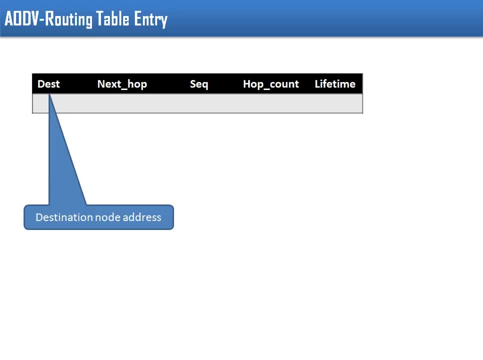 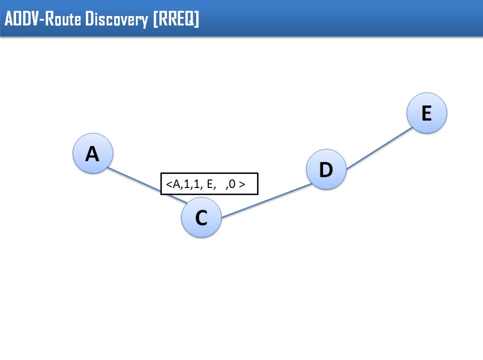 update this packet so every node maintain this information in the table. so these table, we are considering only some few column here: destination, next hope sequence, number, hope count and lifetime when C will received this packet. C would know this packet is actually coming from A and this packet came on this interface. okay, this is connected the using this. 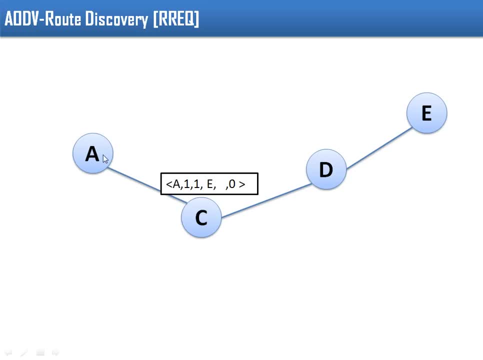 interface. it is connected to A, so it would know this packet is coming from A- a, So it will create an entry in the routing table. What is the entry? If any packet coming to C for destination A, C should transmit that packet in this direction? 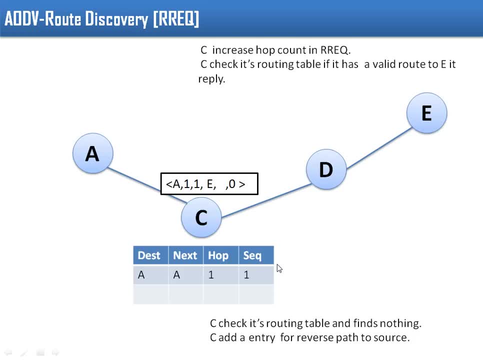 So it will create this entry in the routing table. So this is also known as we are keeping A backtrack for the senders. So this red line, this red arrow is showing actually C, is keeping this information that A is reachable using this path. 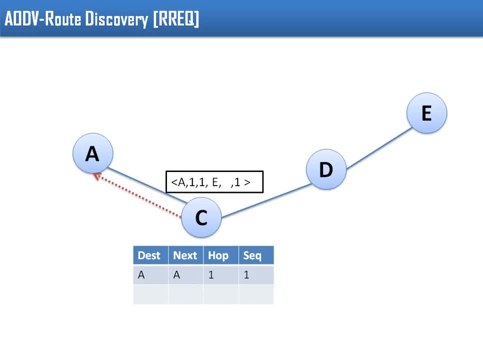 Now C increases the hope count and broadcasts this packet again. D will check that the destination is E. So D will check that the destination is E. D also broadcasts this packet and before that D also make an entry. D will make if this packet is coming from A, from this side. So it would know in order to reach to destination A we have to go to C. 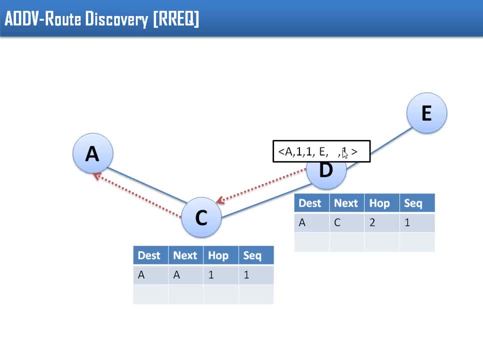 And from here, from the hope count, it will get the hope count information. So this will be the current situation. now D will send this packet to E. Now E will check. This route request packet is actually for C, So now E will prepare a route reply packet and before that E will also create an entry in the routing table. 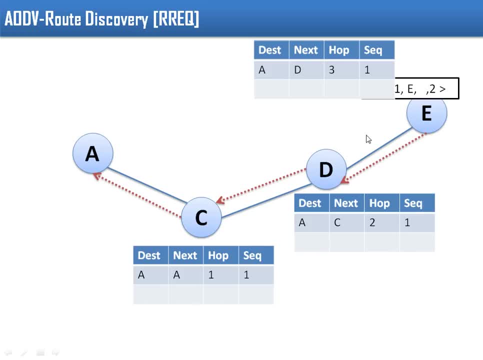 So this red arrow, they are actually keeping track for sender A, how to reach A. So E has prepared a route. reply packet: Sender, Receiver, Destination, Sequence Number, Hope count. So again, hope count is the distance from sender. 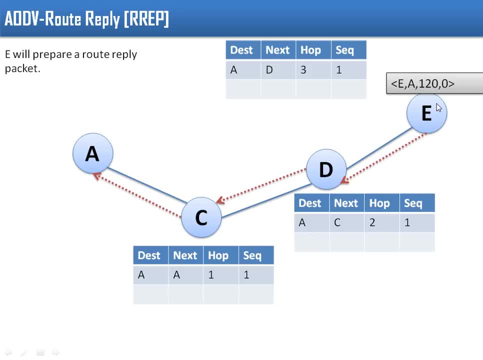 So currently we are on E, So distance from E to E is 0.. E will send this value to D. So now D would know this packet is coming from sender E from this side. So D would know in order to reach E I have to go to here. 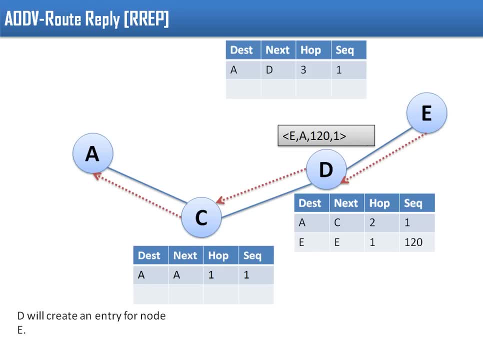 So it will create a entry in the routing table And this entry will say: in order to reach E, Forward the packet to E Hope count is 1.. And this is the sequence number. This is the timestamp At what time destination E has generated route reply packet. 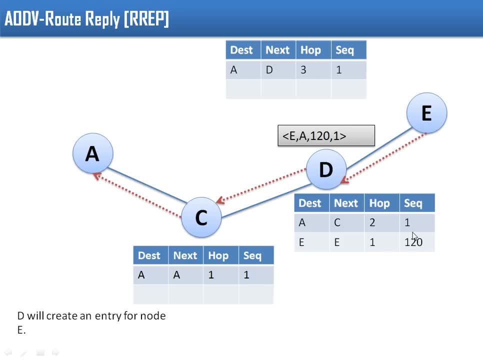 Now D will increase the hope count value and send this to C. C will also make an entry that C will see this packet is coming from E And this packet is coming from D, So it would know. in order to reach E, Hope count is 1.. 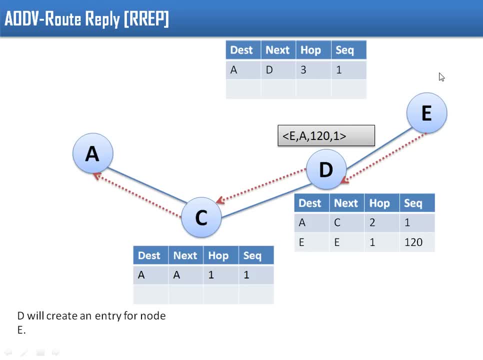 And this is the sequence number. This is the timestamp At what time destination E has generated route reply packet. Now D will increase the hope count value and send this to C. C will also make an entry that C will see this packet is coming from E. 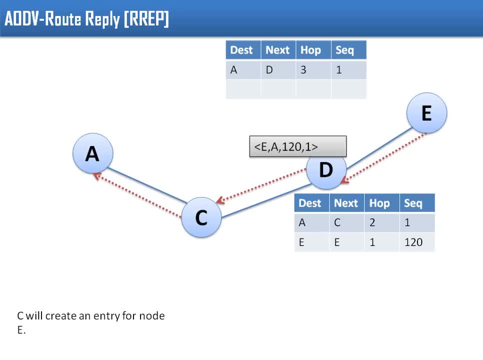 And this packet is coming from D, So it would know, in order to reach E. And this packet is coming from D, So it would know, in order to reach E, this to see. see also make an entry that she will see this packet is coming from. 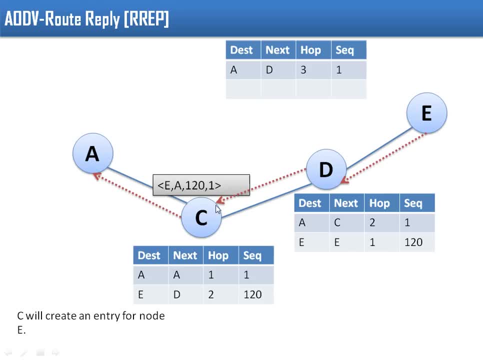 E and this packet is coming from P, so it would know: in order to reach E you have to go to D, so it will create an entry. in order to reach E we have to forward our packet to D. it will take two hop. count and sequence number is 120 and finally,